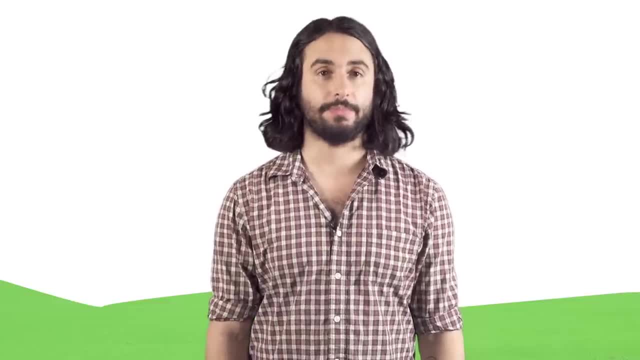 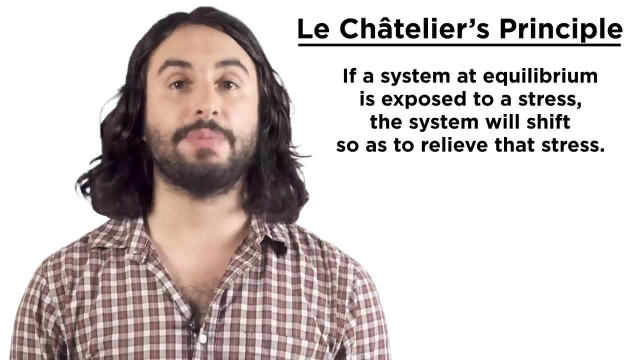 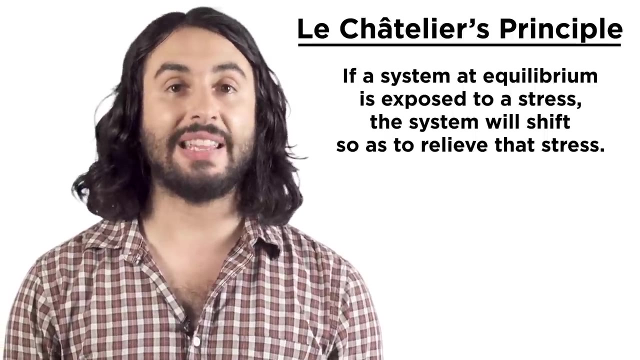 Professor Dave, here let's talk about Le Chatelier's Principle. Le Chatelier's Principle says that if you induce a stress on a system at equilibrium, the equilibrium will shift so as to relieve that stress. So let's see some examples of a stress we could put on a system at equilibrium. 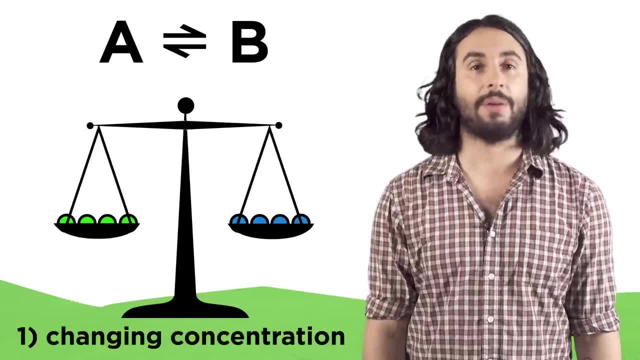 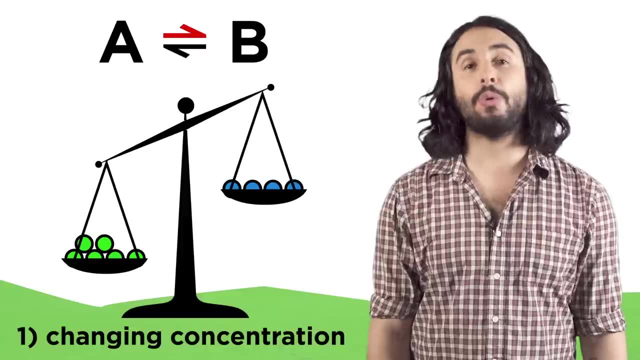 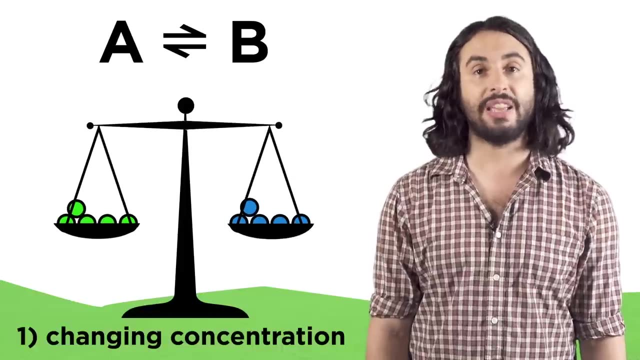 First, we could modify the concentration of any of the compounds. Let's say we add some of this reactant. That will unbalance the equilibrium and the forward reaction will speed up to use up some of the additional reactants, turn them into products and restore equilibrium. 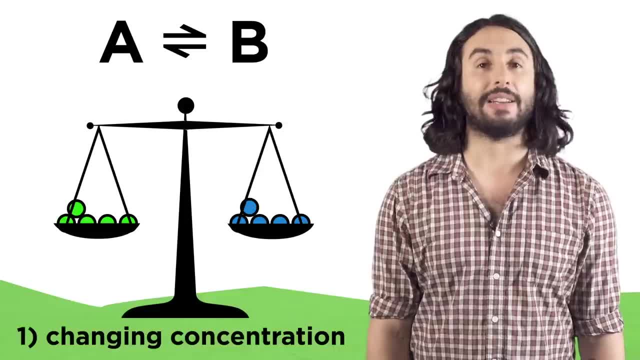 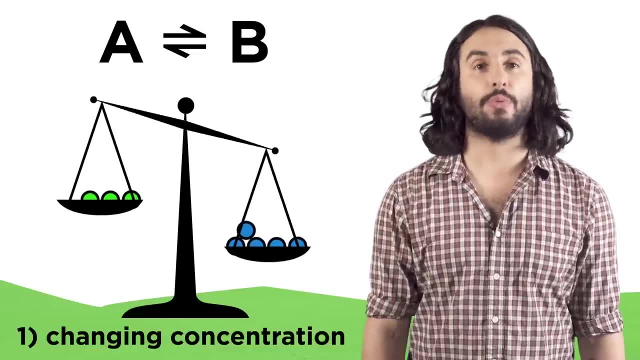 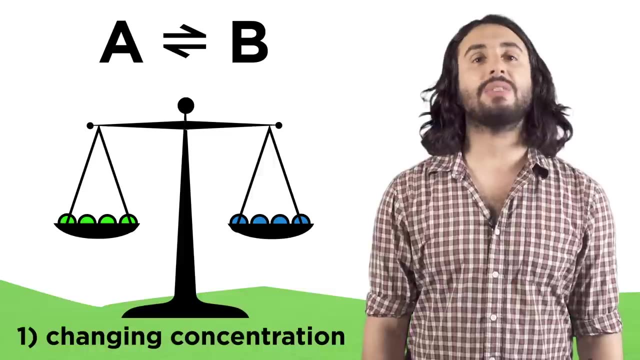 The equilibrium is said to have shifted right. If we add more products, it would shift left. Likewise, if we selectively remove one of the components, the equilibrium will shift to produce more of that species. to restore equilibrium, That is one type of stress we could put on a system. 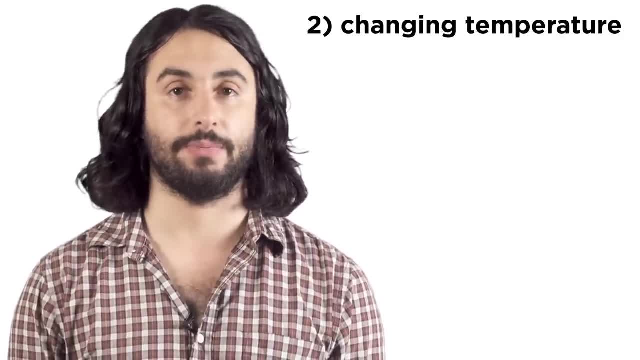 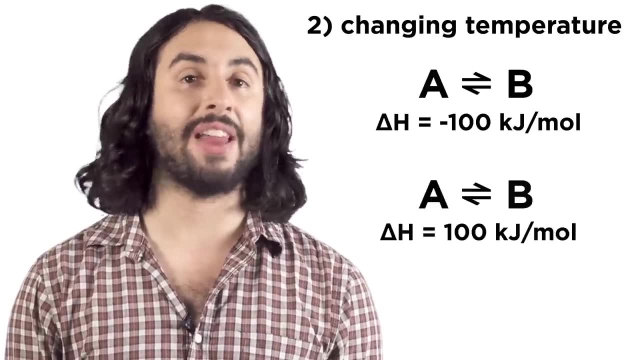 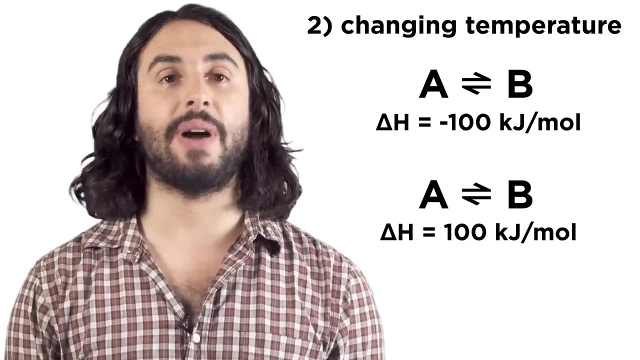 Another stress would be to change the temperature, To see how this would affect an equilibrium. we have to see whether a given reaction is exothermic or endothermic. This tells us whether a reaction absorbs or releases energy and is signified by delta H, the change in enthalpy. 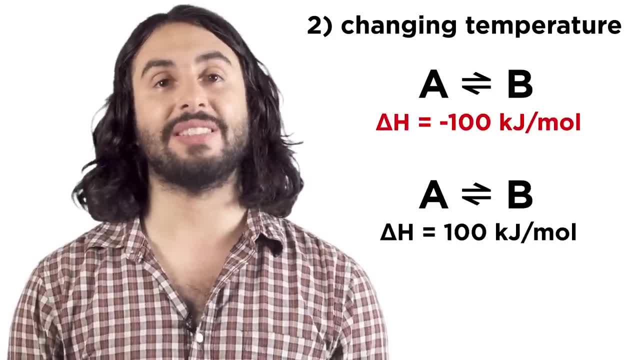 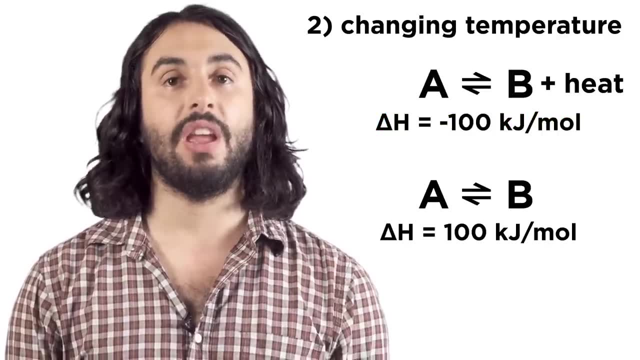 If delta H is negative, the reaction is exothermic and releases energy, So we could think of heat energy as a product of this reaction. If, instead, it's positive, that means it's endothermic and energy must be absorbed for the reaction to go. 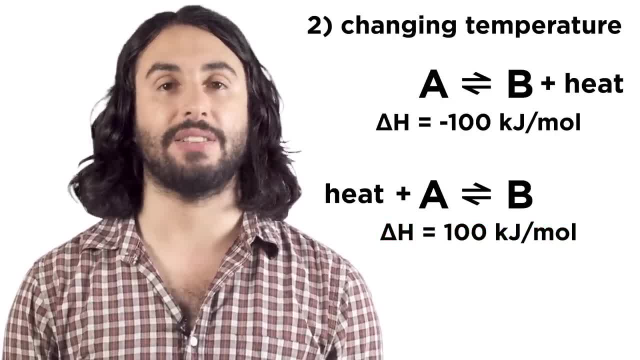 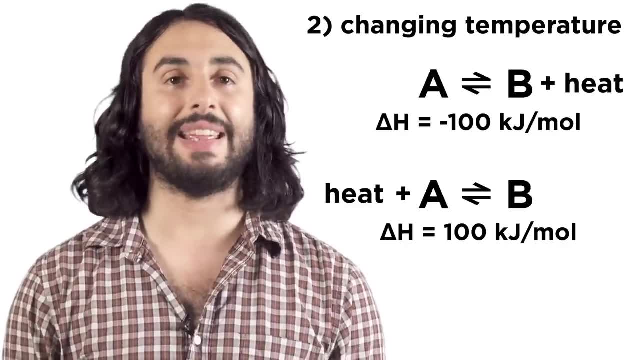 So we could think of heat energy as a reactant in that scenario. Once we translate thermochemical data in this way, we can treat the word heat as just another substance involved in the reaction. Higher temperature means more heat, so things will shift. 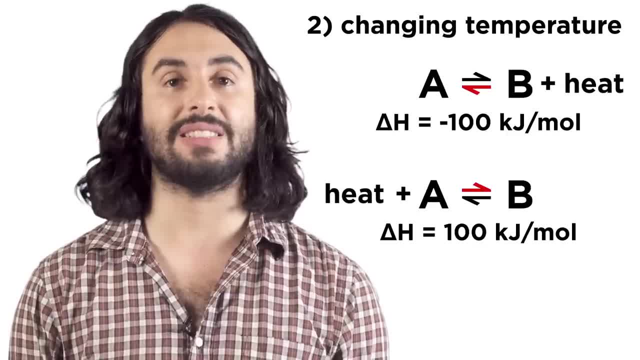 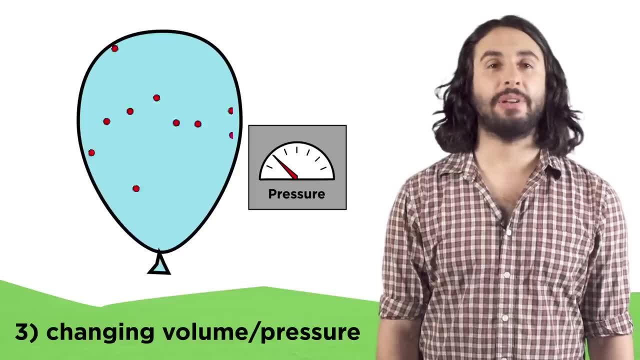 So things will shift to the other side: to use up some excess heat and relieve the stress. Cooling it down would have the opposite effect. The third stress we can examine is changing the volume or pressure. Let's say the equilibrium involves gases in a balloon.